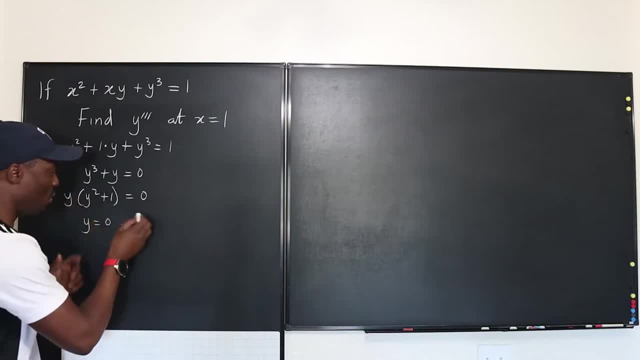 number. there's no real value for which this will ever be 0, or we can just say that y squared equals negative 1.. You can see that that implies 0.. Let's do that again. So that's the same thing that we did with the previous equation. So 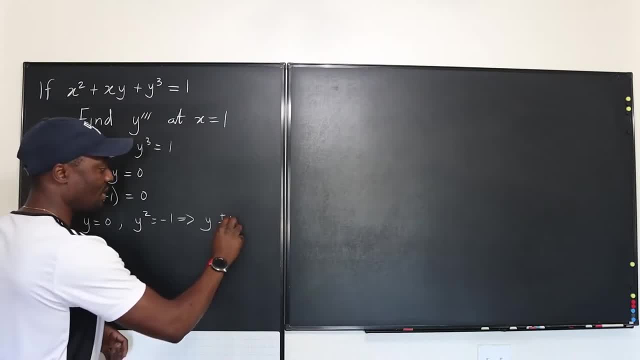 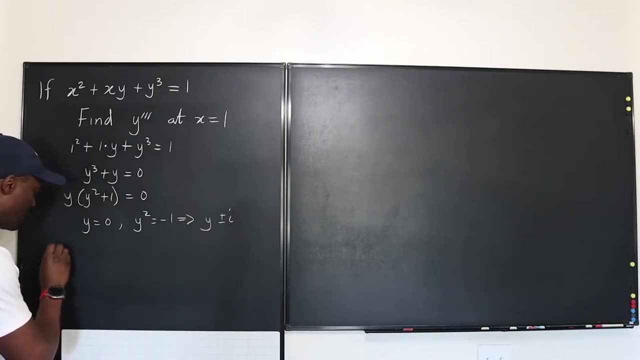 now we're going to get y minus y, squared, plus or minus the square root of negative 1, which is i. but we don't want to deal with this right now, so this entire part is not relevant. So the point that we're dealing with so point is the point where x equals 1, and y equals. 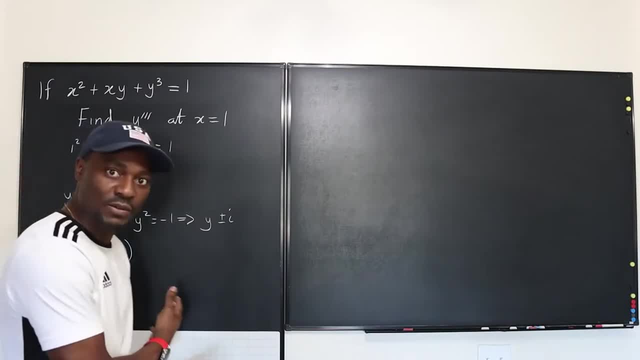 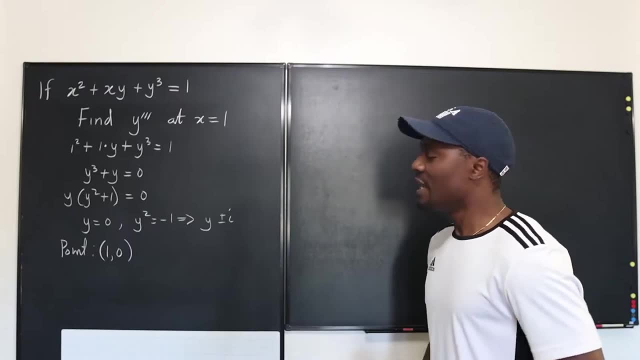 0.. It's the point. So at least we've gotten the 1st point. so we know that when x is 1, y will be 0.. Okay, Now let's start our differentiation. Okay, We haven't differentiated, we just secured the point, and you see why I dismissed this. 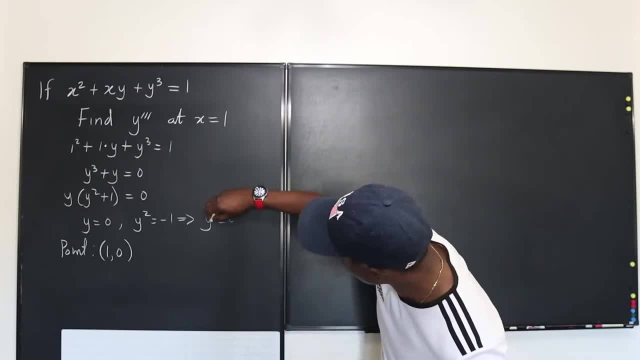 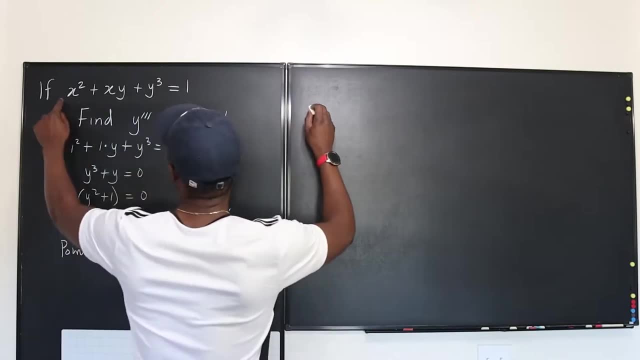 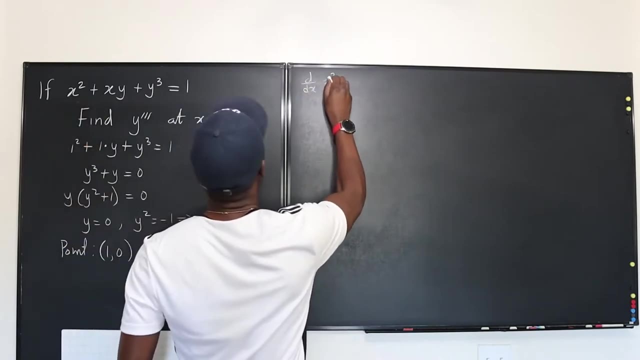 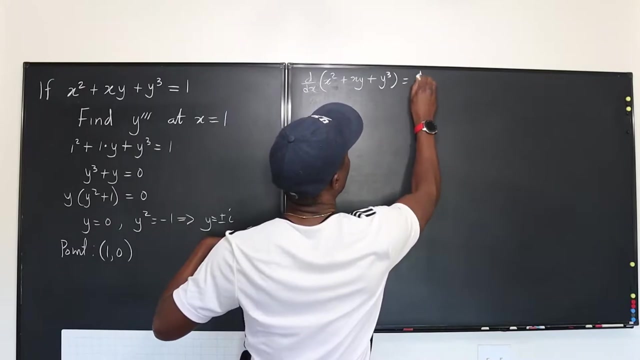 because this is going to be not real. What did I do here? y equals plus or minus i. Okay, now let's go here and start our differentiation, If we differentiate both sides. so we're going to start. we say: ddx of x squared plus xy plus y cubed equals ddx. 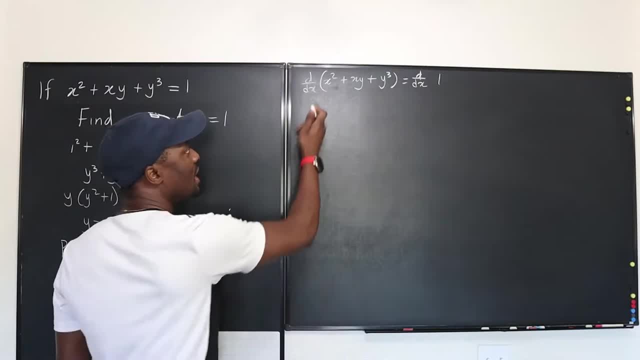 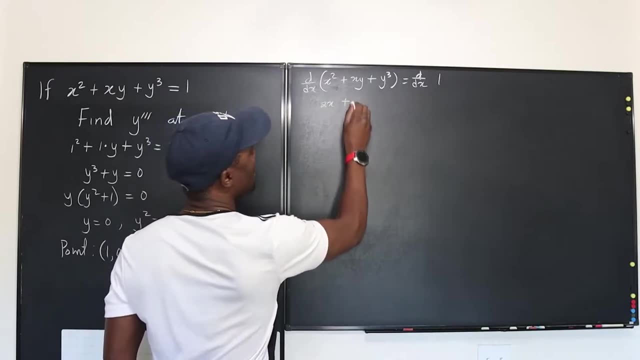 Of 1.. Okay, so we're differentiating both sides. Now, if we apply our simple differentiation power rule, this is going to be 2x and this is going to be plus. Now, this is the product of two functions. both of them are functions of x. 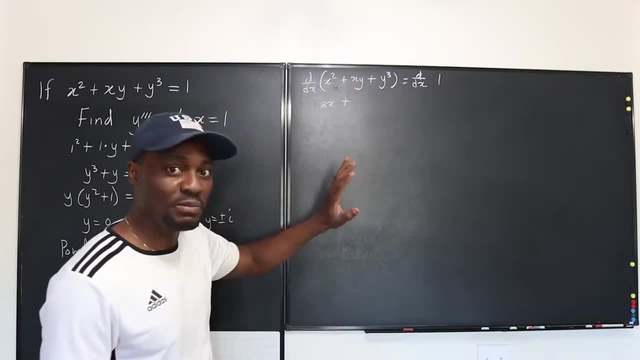 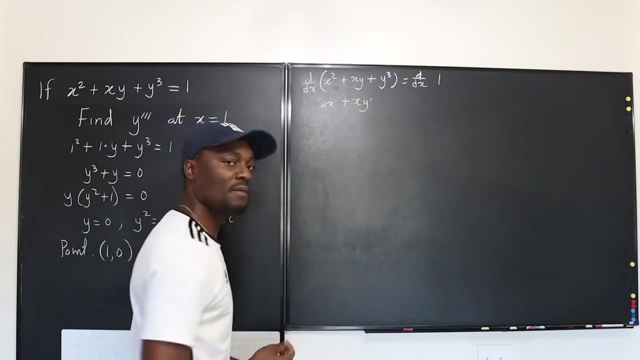 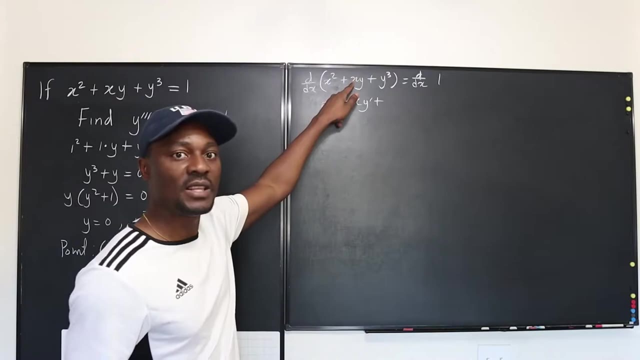 So we're going to apply the product rule. So remember the product rule: keep the first, differentiate the second, Then plus Now, differentiate the first, keep the second. To differentiate this, you get 1, but you have to keep this. 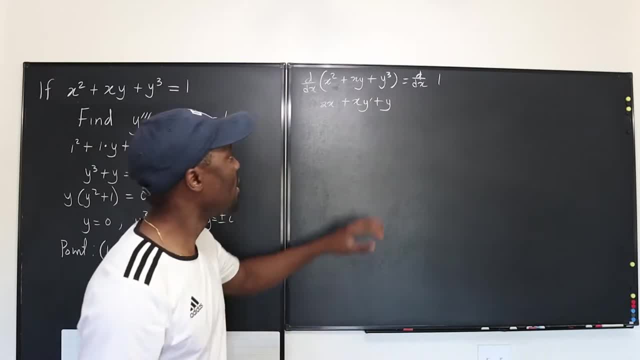 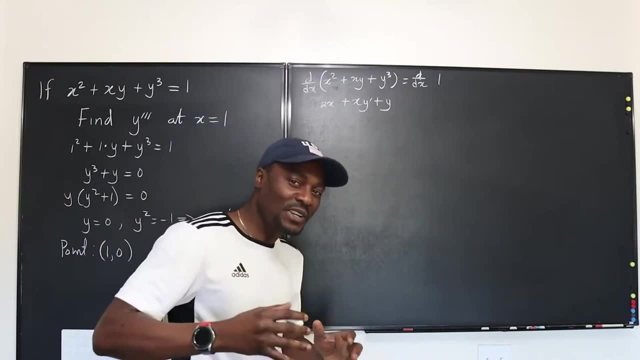 So it should be 1 times y. So that's all you get. Now we go to the last one. This is y cubed. Well, remember that y is more like the function of x is a function of x. 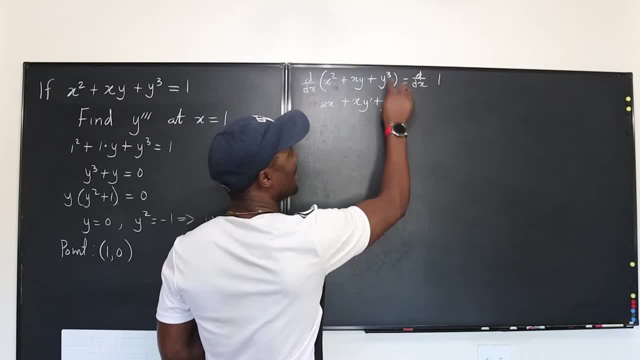 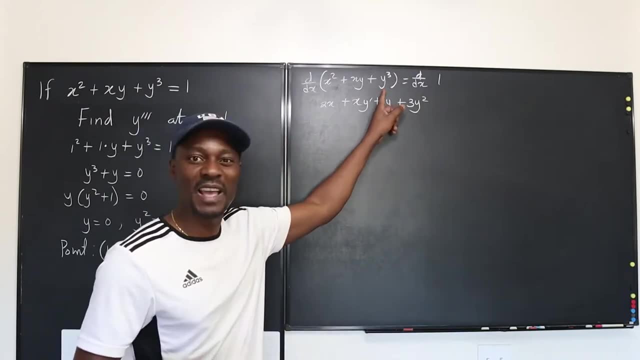 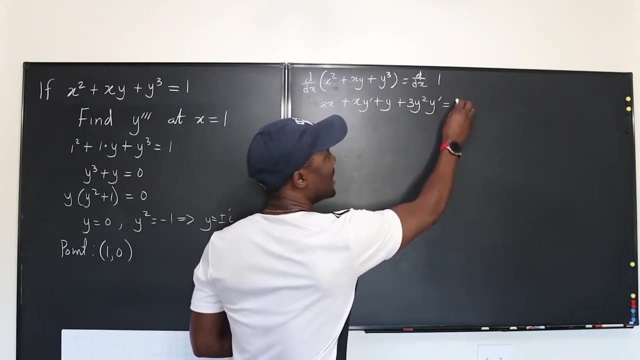 So you differentiate the outside first, so that's going to be plus 3y squared. But because, Because y is a function of x, you have to differentiate the inside, which will be y prime, y prime, And if you differentiate a constant you get 0.. 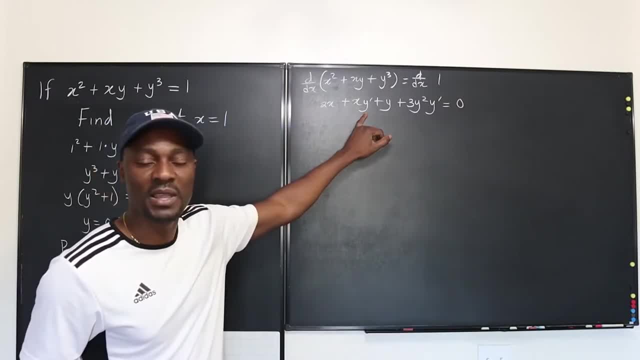 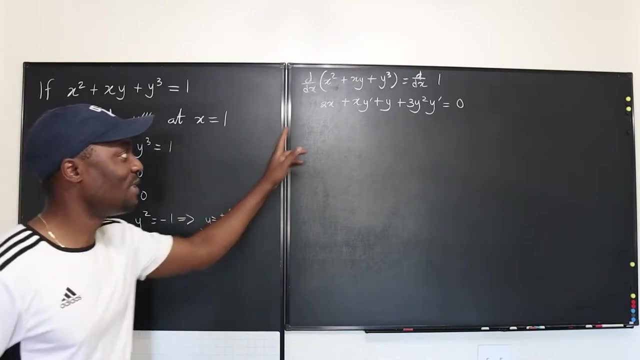 So this is what you get, and this has given us y prime. What's the value of y prime at this point? Well, you don't need to worry. Just plug in these two values there and then you're going to get your y prime. 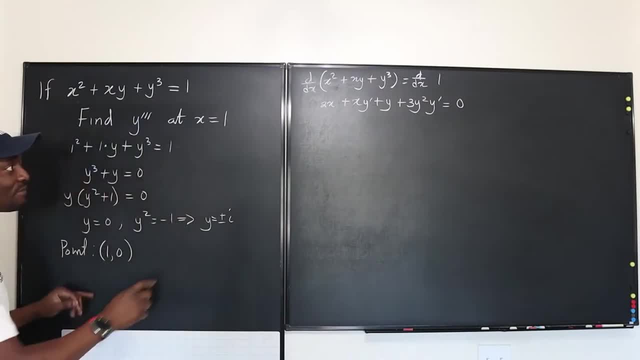 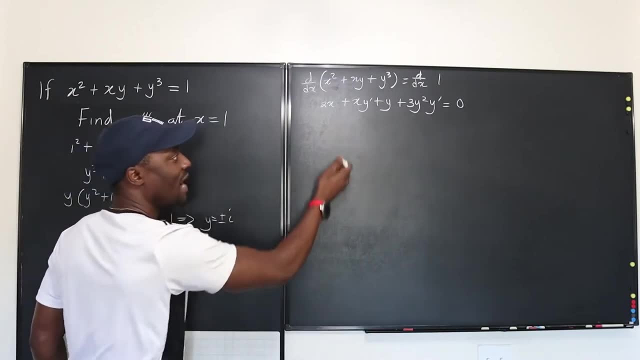 Okay, let's do it here. So we're going to say 2x plus xy, So we're going to plug in these two numbers for this. I don't want to write it here because I need, You know what. 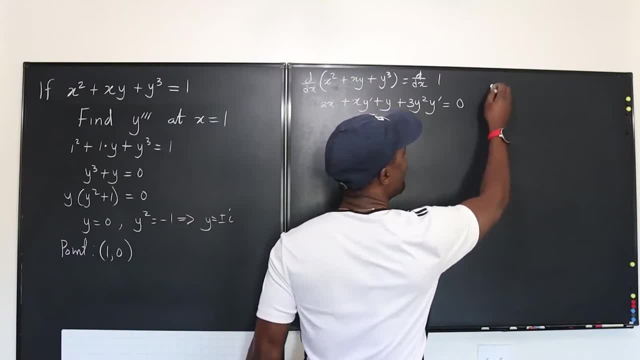 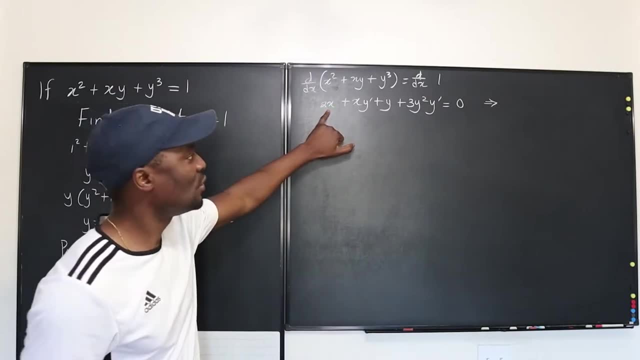 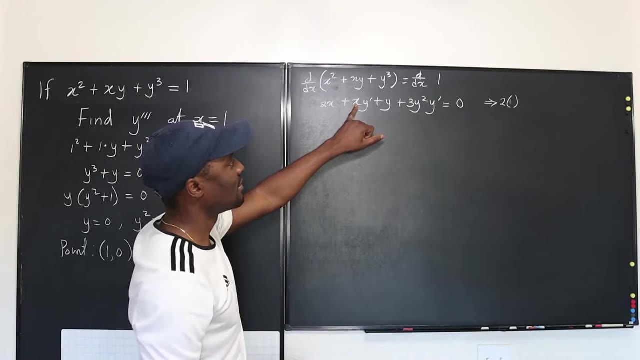 I can write it on this side, So let's do this. This implies Okay, If I put 1 here for 2, so it's going to be 2 times 1 plus 1 times y prime plus 1 into. 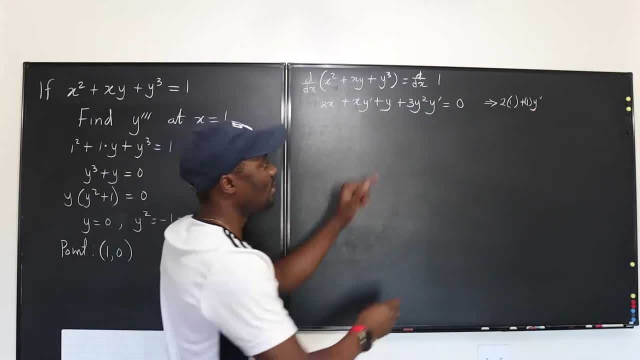 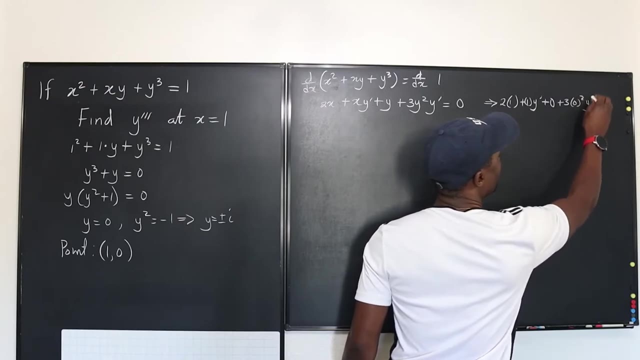 y prime. okay, plus y, but y is 0.. You see that Then if I go here, this is going to be 3 times 0 squared y prime. That would be plus 3 times 0 squared, and then you have y prime will be equal to 0.. 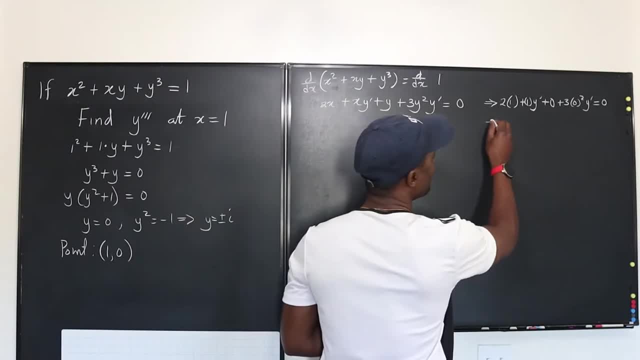 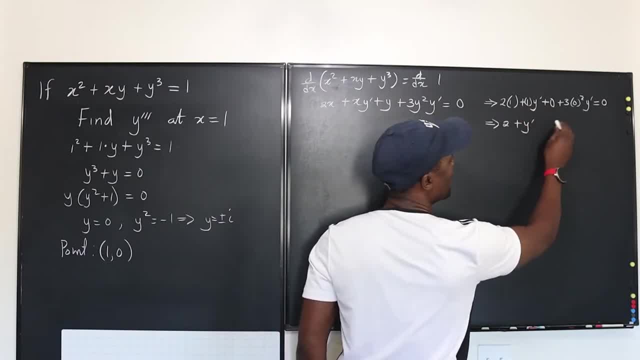 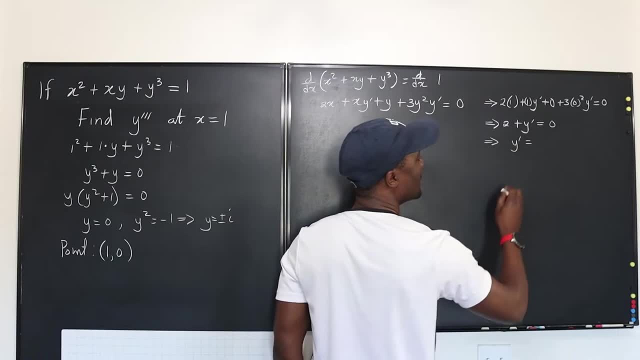 This is going to be y prime and this is going to be 0, 0, 0, 0.. So that tells me that y prime is equal to negative 2.. So now I have another number that I can add to this. 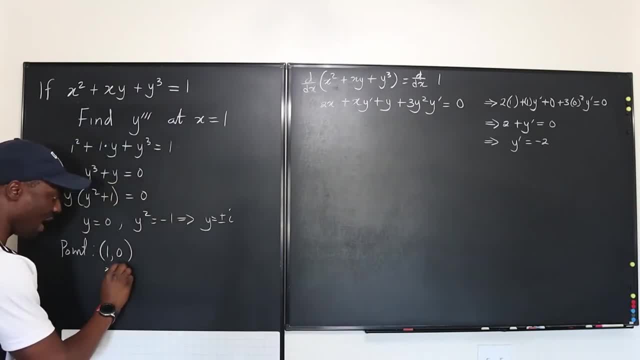 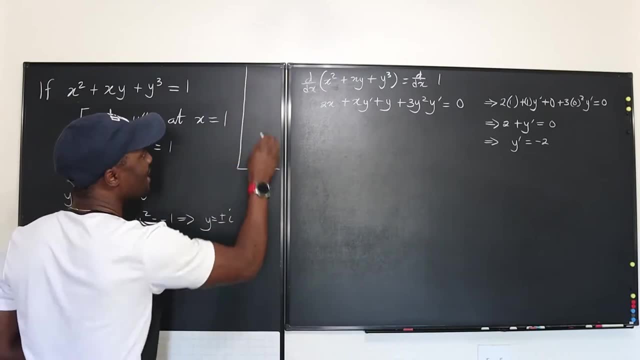 So the point is this: This is x, This is y, Or I can just make a list somewhere here. okay, just to make life easy, Say x equals 1.. y equals 0.. y prime equals negative 2.. 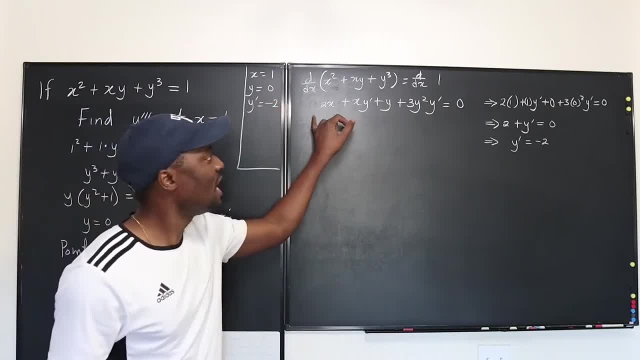 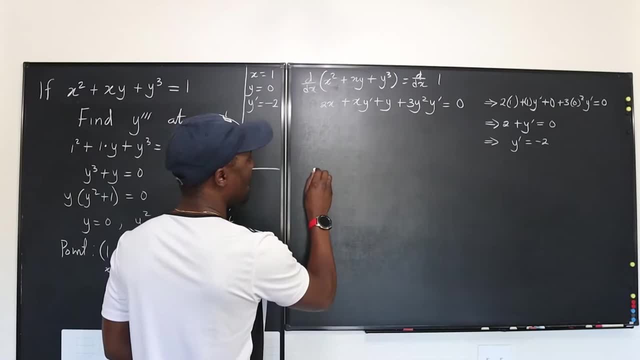 Okay, Let's go to the second differentiation. Now we're going to differentiate this again so we can get to y prime prime, Okay. So if we differentiate this, you have 2, just 2.. Let's move up. 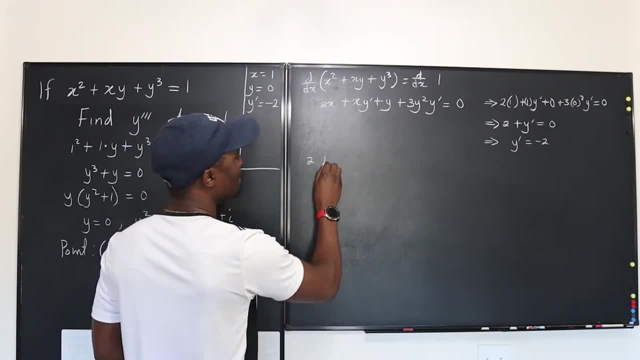 We have 2, and then if we differentiate this, we apply the product rule again. You have to be careful, Apply the product rule, Remember keep 2.. Keep the first, Differentiate the second: x, y, prime. 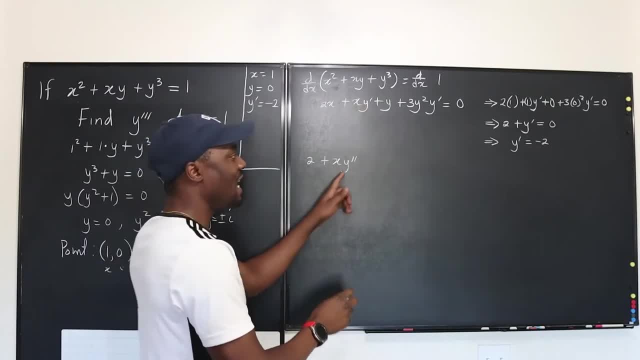 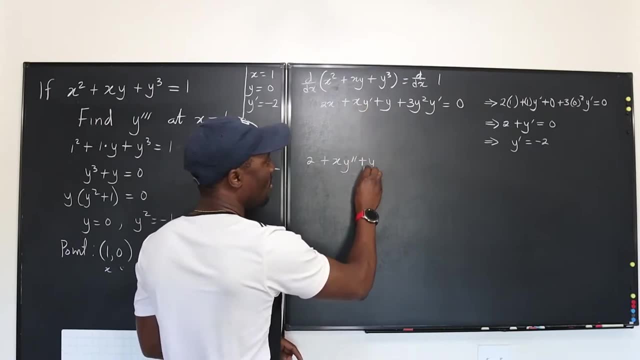 Prime. Keep the first, Differentiate the second, Then differentiate the first, Keep the second, Differentiate the first, you get 1.. Keep the second, y prime. Okay, Now we move onto this one Plus. if you differentiate y, you're just going to get y prime. 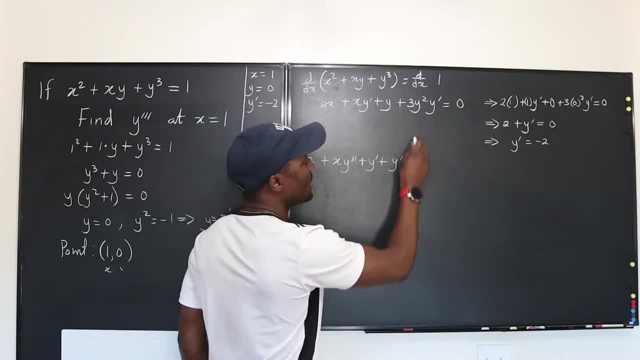 Okay, You go to the next one. Differentiate this one. now What we're going to do is just write the 3 and multiply by 4.. Okay, by when we differentiate this. So remember the rule: keep the first, differentiate the second. 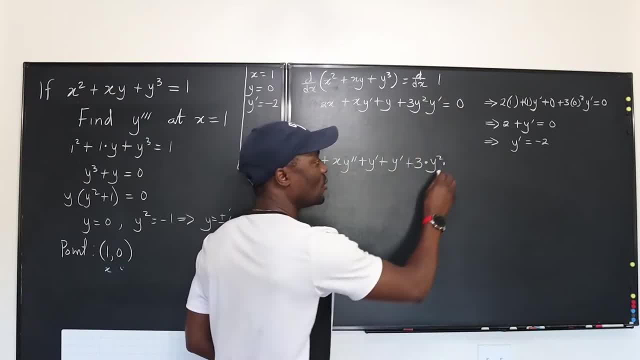 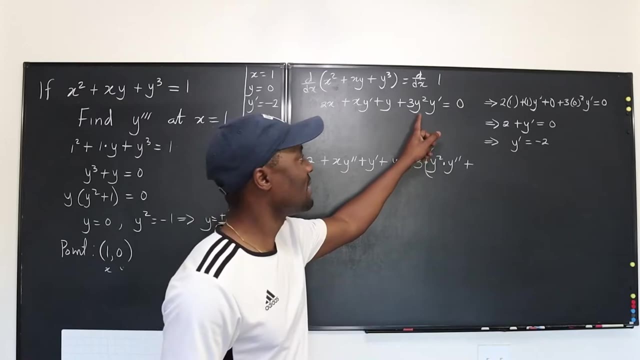 So that's going to be y squared times. the second will be y prime prime now plus differentiate the first. So we're going to different. let's put this here because we're not done. The three is outside. Okay, We're going to differentiate the first and then keep the. 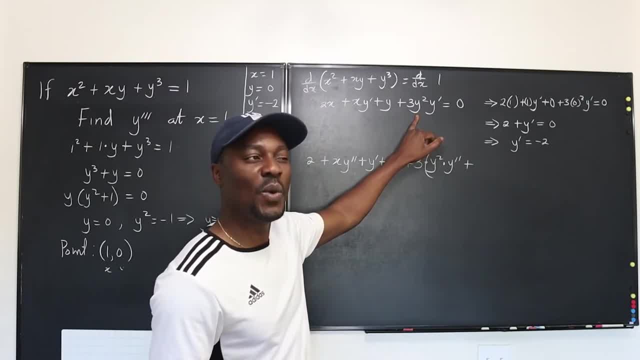 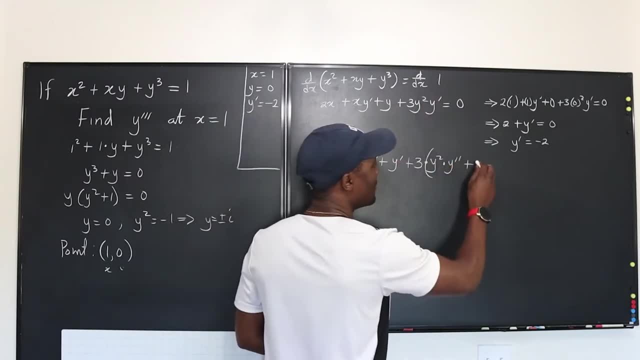 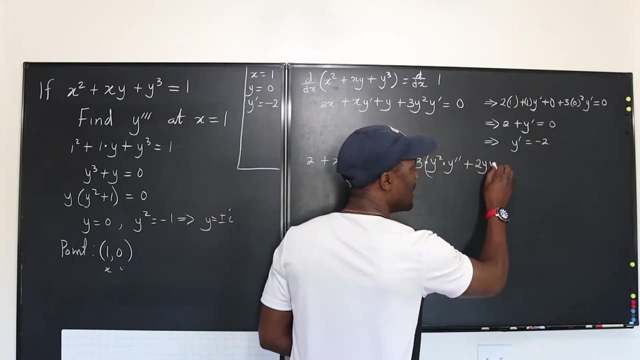 second, How do we differentiate y squared? It will be 2y times y prime, Remember, because this is a function. so we'll differentiate first the outside 2y, then we multiply it by the derivative of y, because it's a function of x, y prime, Then we multiply it by what we have here, Oh, y prime. 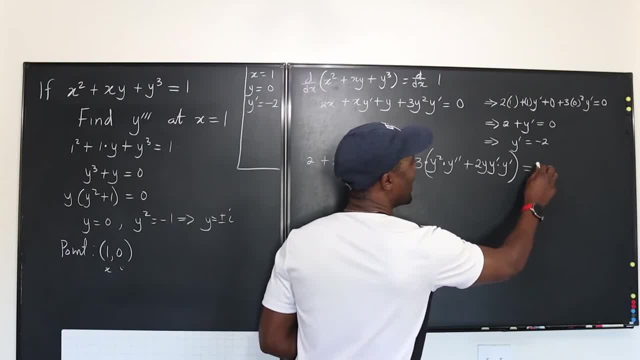 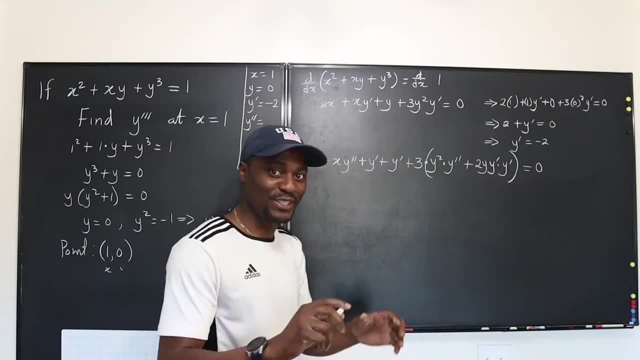 You see, where I said it's going to get messy, And on the right-hand side you have zero. So at this point it's important that you clean things up, because you still have one more differentiation to do. So it's recommended that you clean things up. So I'm going to write 2 plus this is going to be: 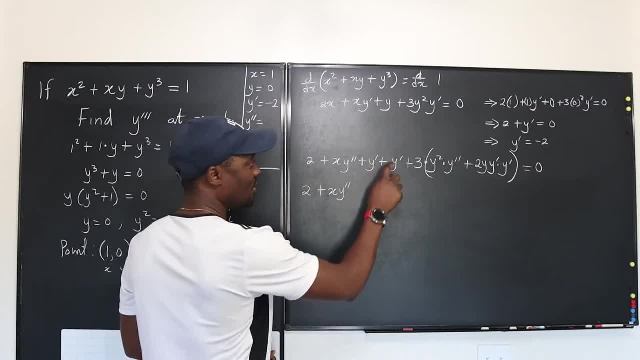 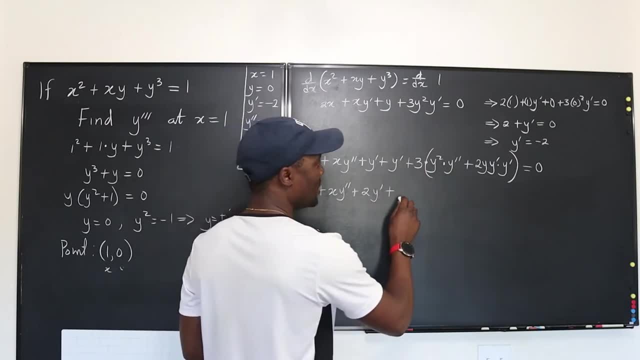 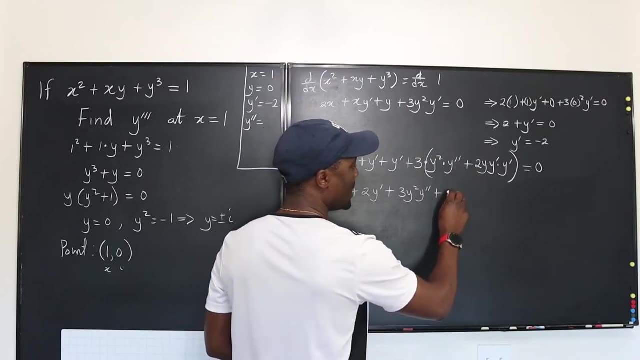 x- y prime prime. I'm going to add these two together. That's going to be 2y prime plus. I'm going to distribute this. This is going to be equal to 3y squared y prime prime plus. 3 times 2 is going to be 6,. 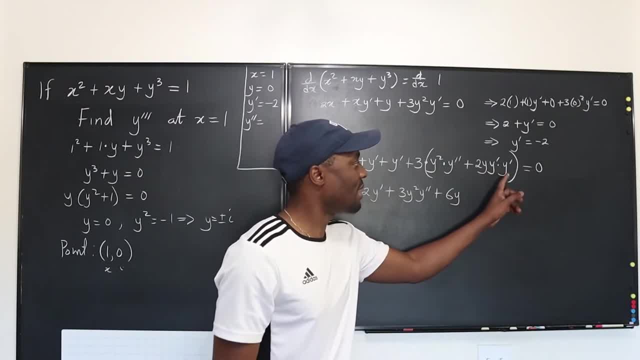 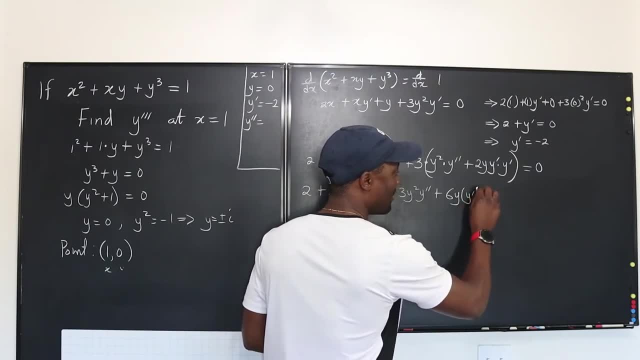 y. Well, you see, this is y prime times y prime. so it's going to be y prime squared. Be careful, It's going to be y prime squared equals zero. So that's what we've got Now at this stage. 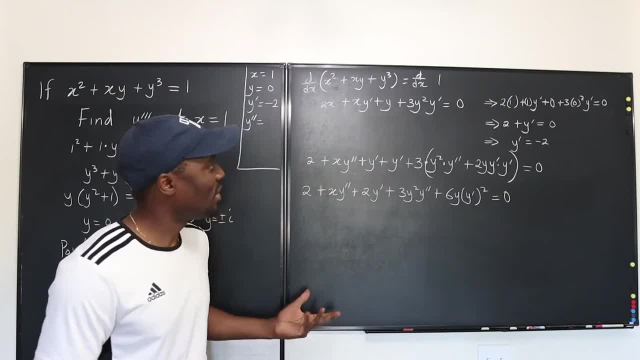 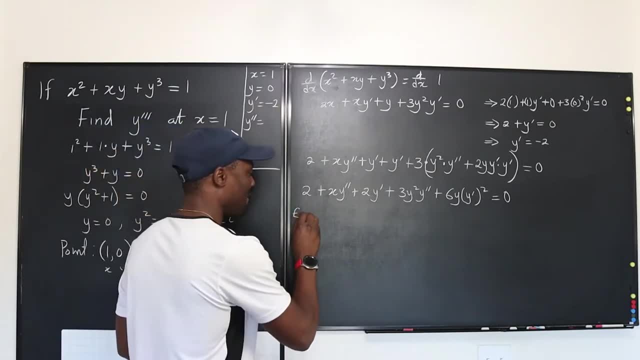 I can evaluate. okay, I can evaluate. plug in x equals 1, y equals 0, y prime is negative 2, and see what happens. So let's evaluate. okay, I'm evaluating. So what I did here is what I'm going to do here, but because I don't have enough, 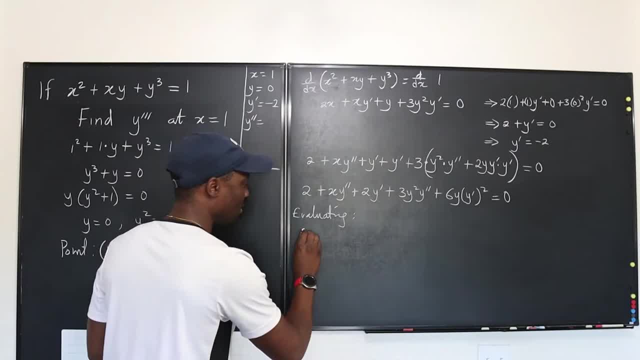 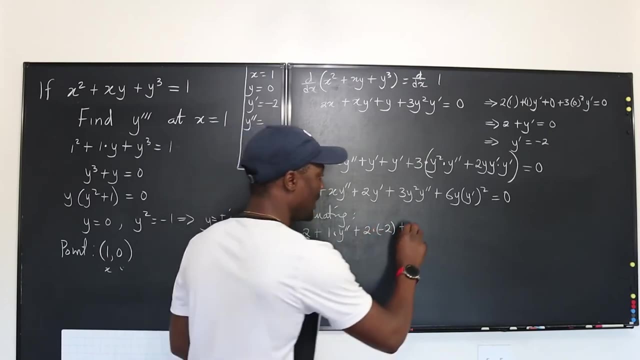 space. I'm just going to do it here. So this is going to be 2 plus 1 times y prime prime plus 2 times what is y prime Negative 2, okay- Plus 3 times what is y squared or y zero, Zero squared. 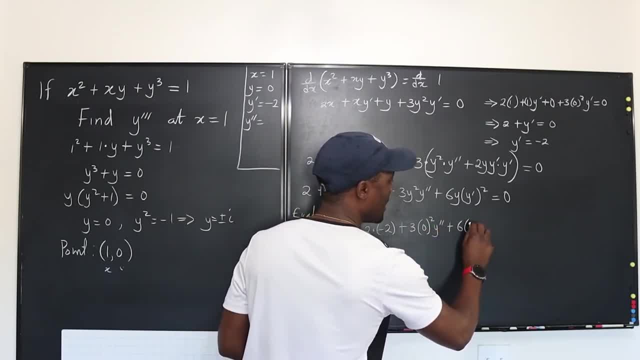 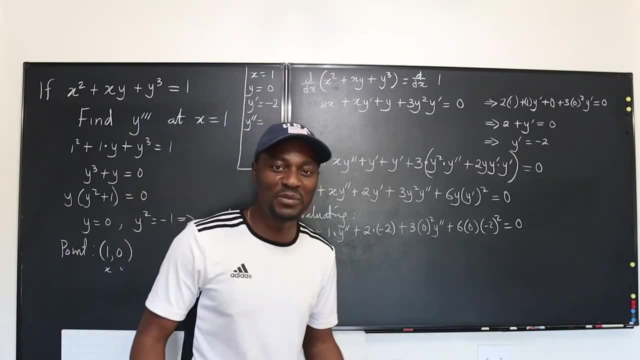 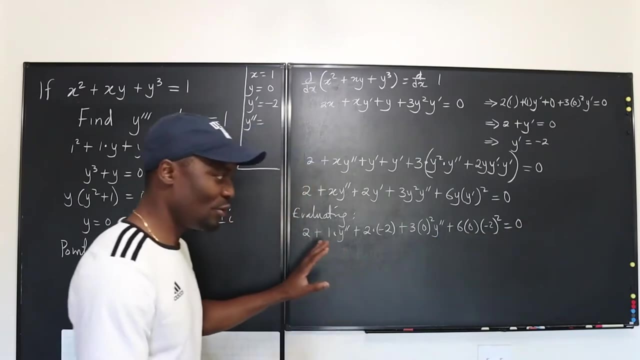 Y prime prime plus 6 times 0 times negative, 2 squared equals 0.. So usually there will be some easy number for you to work with, okay, So this zero will delete this entire term and this zero also here will delete everything. So you notice that what you're left with? let me just put it. 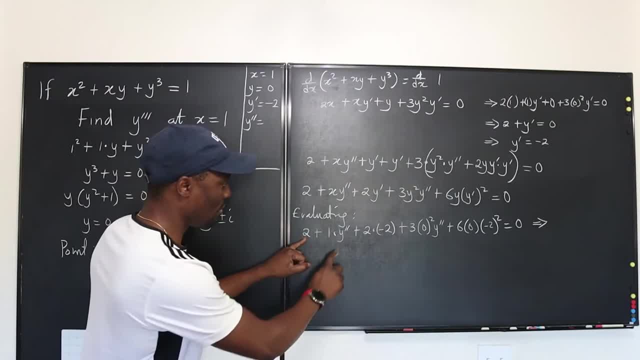 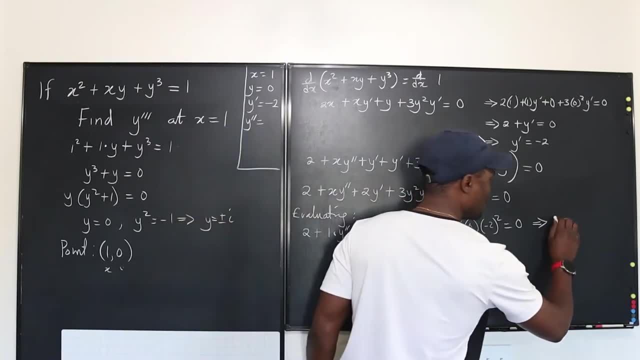 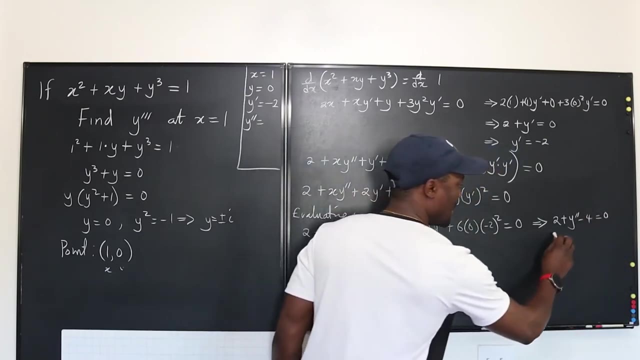 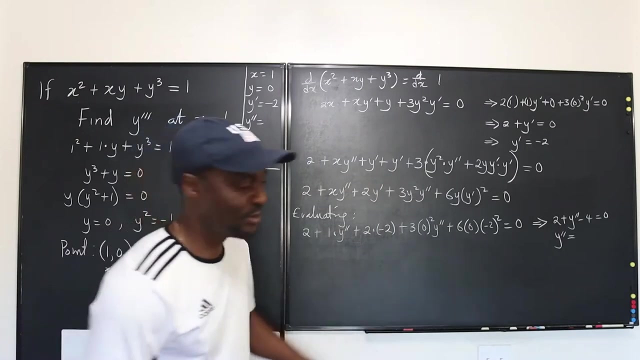 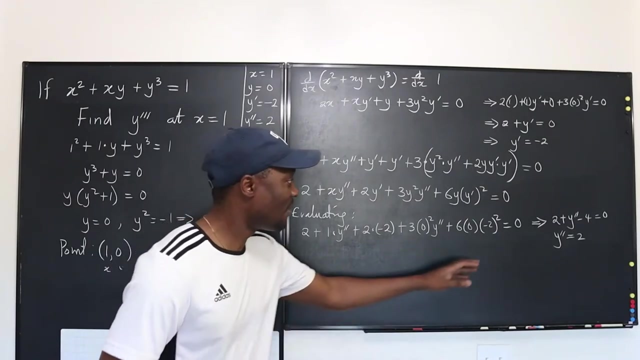 here. This implies that 2 plus y prime prime plus- sorry, minus 4.. Yeah, So we have 2 plus y prime prime minus 4 equals 0. That tells me that y prime prime is equal to 2.. Okay, So I can go here and add to the list. Okay, Let's do the final run Now that we have. 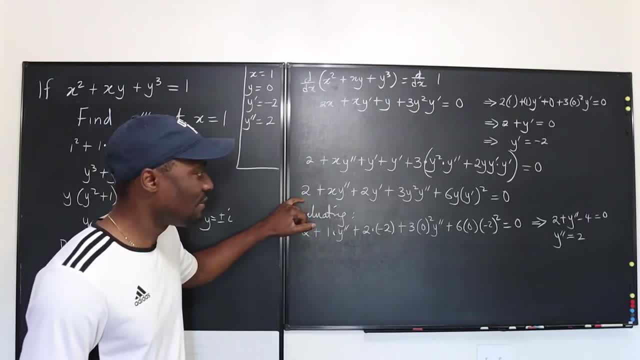 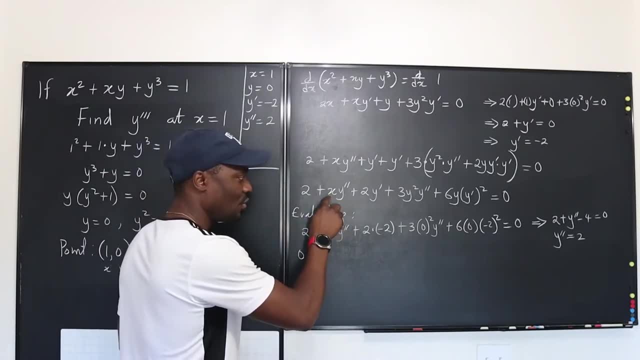 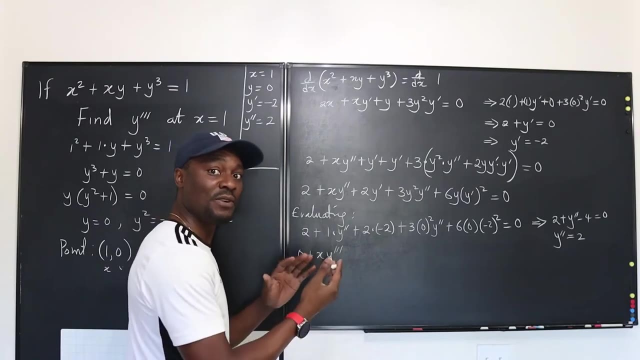 all of these numbers here. let's differentiate this function one more time, carefully. We differentiate this function one more time. We differentiate this function one more time. We keep the first, differentiate the second And then you reverse it. You differentiate the first. 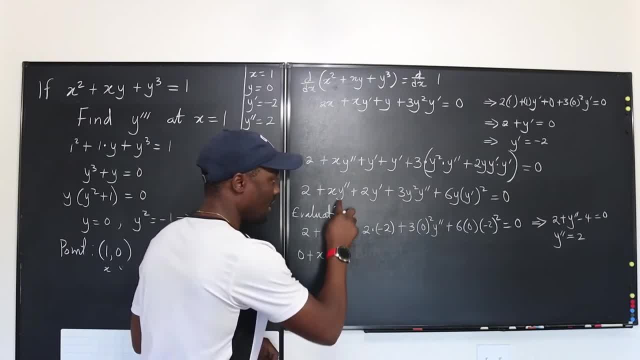 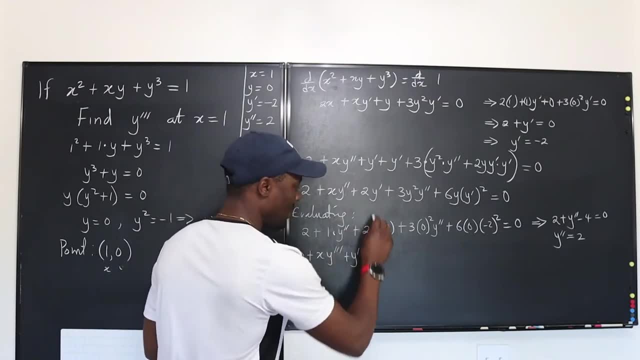 keep the second. If you differentiate this, you get 1.. And then you keep the second: y prime prime. We're done. We go to the next one. Well, you just differentiate this, It's going to be 2y prime prime. We go here. We keep the first, differentiate the second. 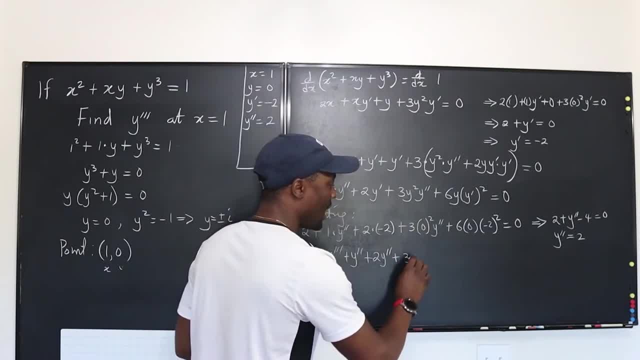 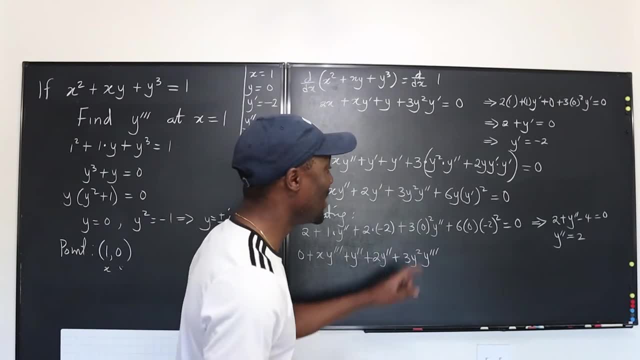 So that's going to be plus 3y squared. Differentiate this: That's going to be y, prime, prime, prime. Whoa, that's cool. And then you reverse the process. I'm just going to repeat the exact same thing. 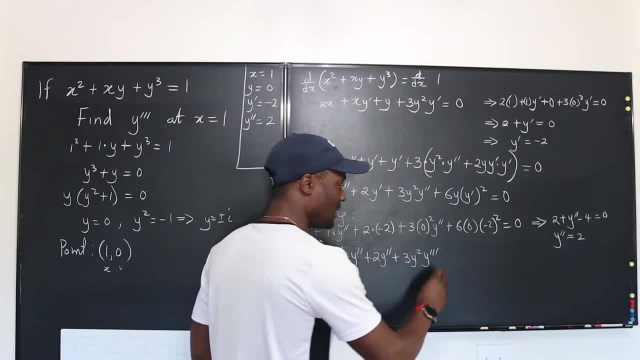 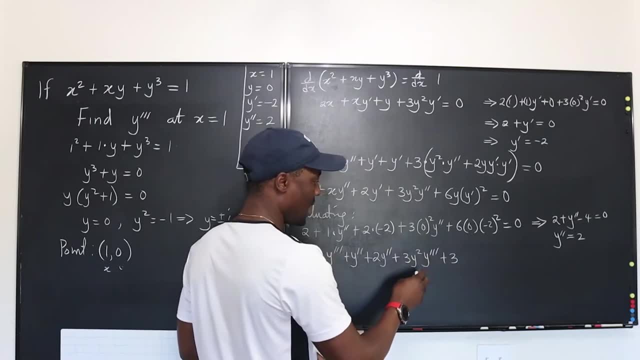 but this time I'm going to differentiate the first and keep the second, So that's going to be plus 3.. Oh, if you differentiate the first, it's going to be 2 times 3. And that tells you it's going to be 6.. 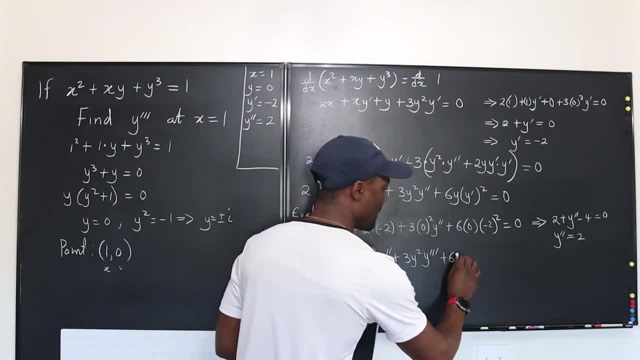 So I'm going to change this to 6.. Okay, 6y, But because this is a function of x, remember it to be times y, prime, And then you keep the second y prime, prime. So this could be the most confusing of all, okay. 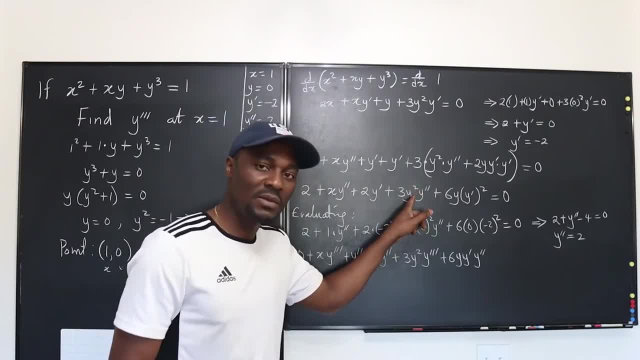 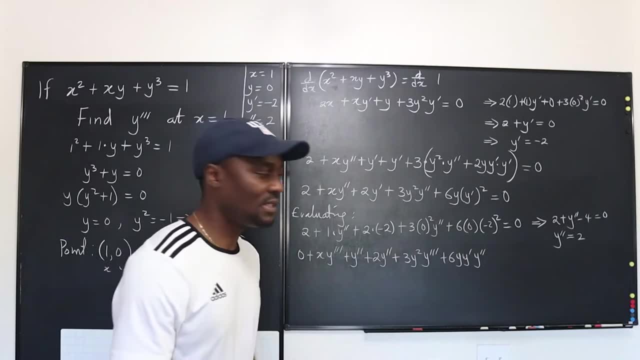 So this is going to be 6y, then y prime, because that's the derivative. It's 6y y prime, That's the derivative of 3y squared, And then you just keep the second. So we're done with that. 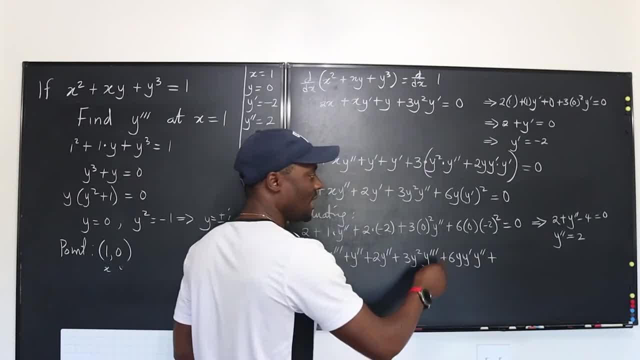 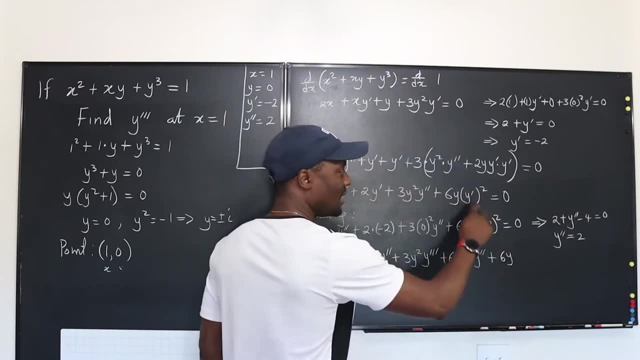 Now let's go to this. This final one is going to be: you do the same thing. We're going to keep the first, differentiate the second, So it's going to be 6y. If you differentiate this, it's going to be 2y prime. 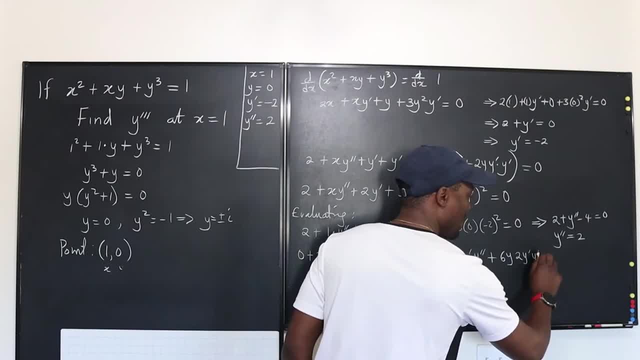 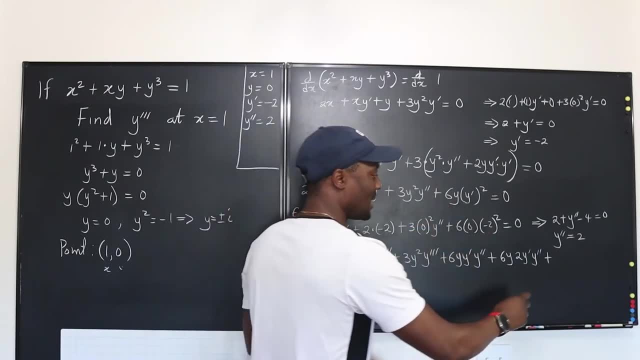 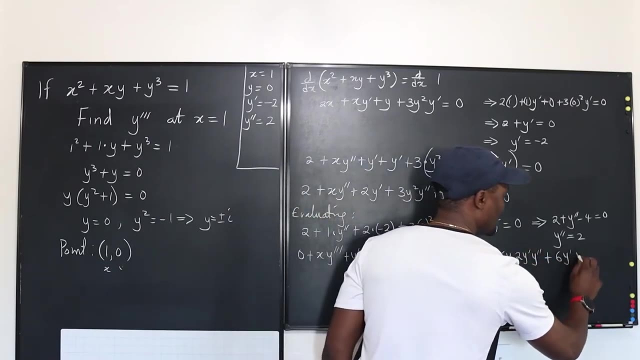 But you have to differentiate the inside y prime prime Interesting. Plus, you differentiate the first and keep the second. That's easier. If I differentiate y, it's going to give me y prime And then I keep the second, which is y prime squared. 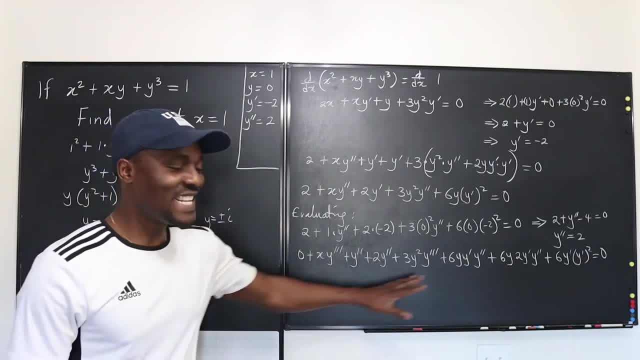 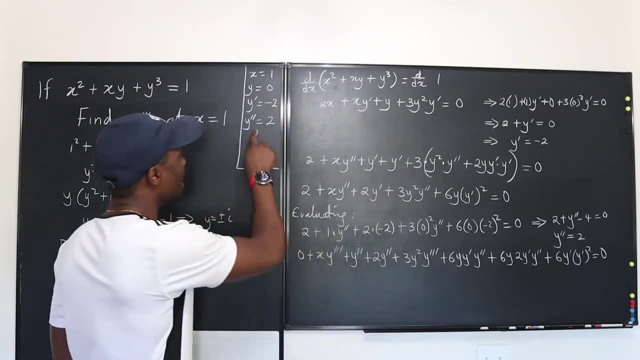 And the end of it is 0. So let's clean this up and then we substitute. Or, before we even clean this up, start looking for all the terms that contain y, Because you're going to get a 0 from there and we don't want to carry that over, okay. 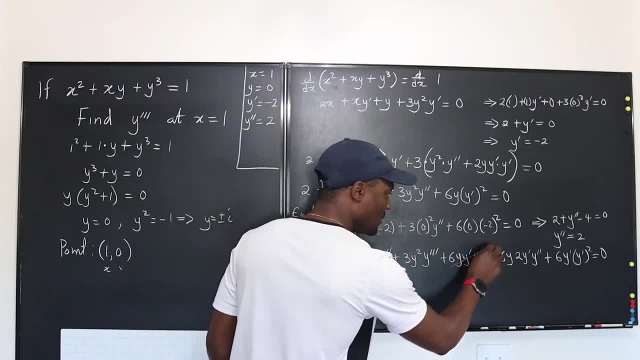 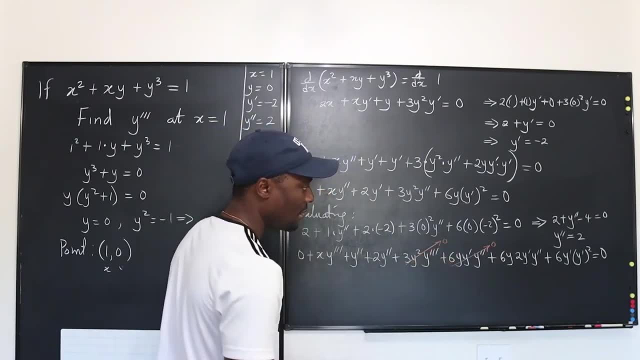 So it's a safe way to say: this is going to go to 0, okay. If it contains y, it's going to become 0.. This is going to go to 0.. This is going to go to 0, okay. 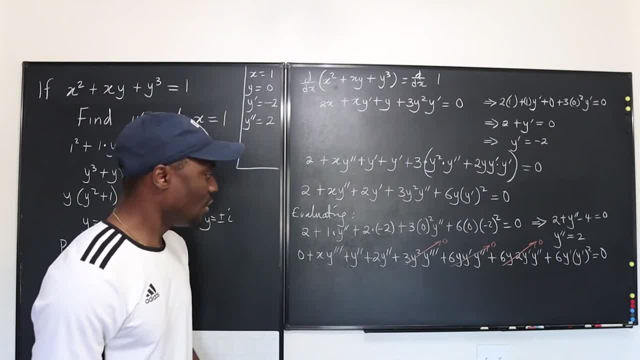 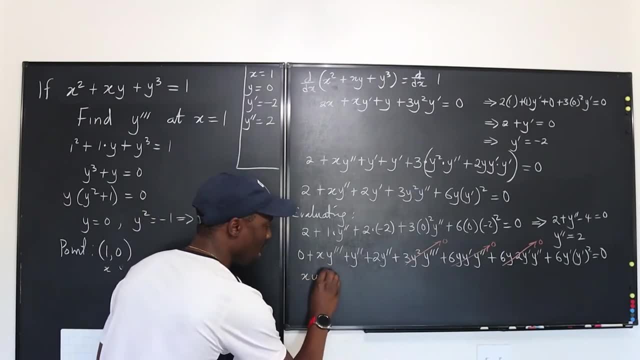 I don't even care right now. Okay, so the rest of the terms do not contain 0.. Now we can write them out. So this is going to be x, y, prime, prime, prime, Plus we can add these two together. 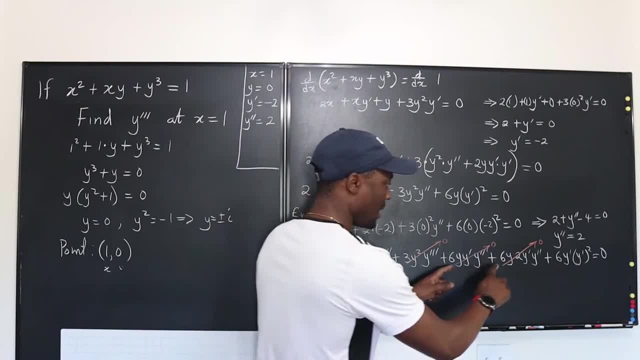 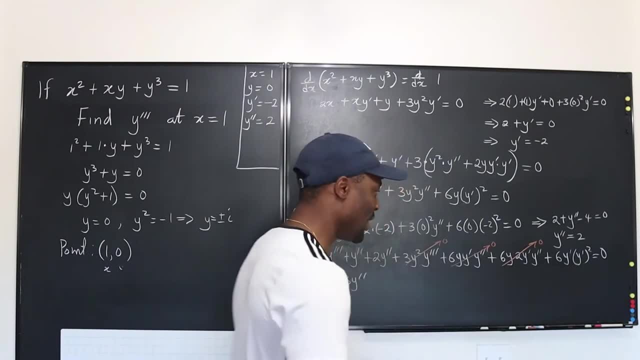 It becomes 3y prime prime And oh, this is the only term left- And you notice that this is y prime times y prime squared. That gives you y prime cubed. So we can write: plus 6y prime cubed equals 0.. 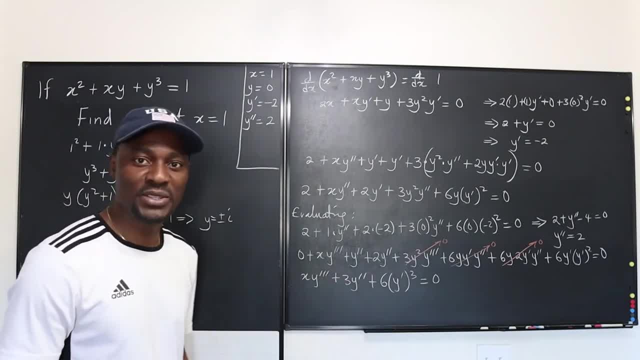 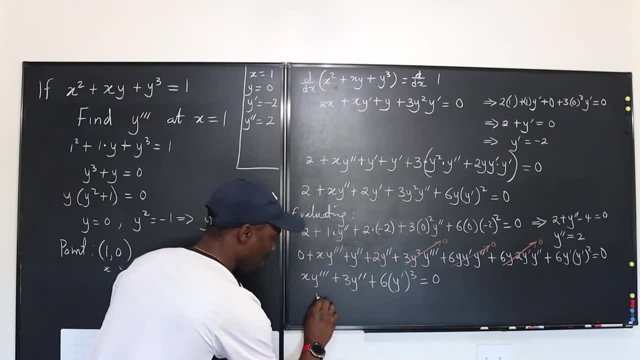 So let's find this guy by just substituting the other numbers and we're going to see what we get. So let's substitute. We have 1 here, so this is going to be y, prime, prime, prime, plus 3 times. 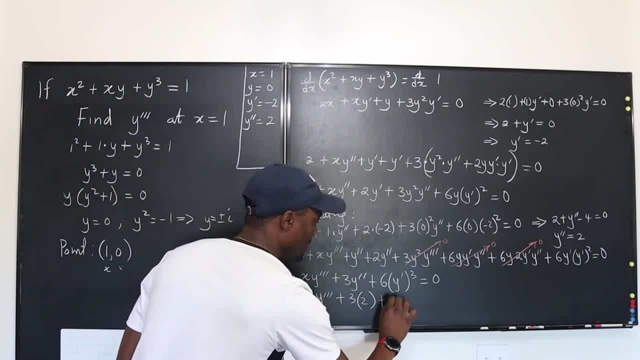 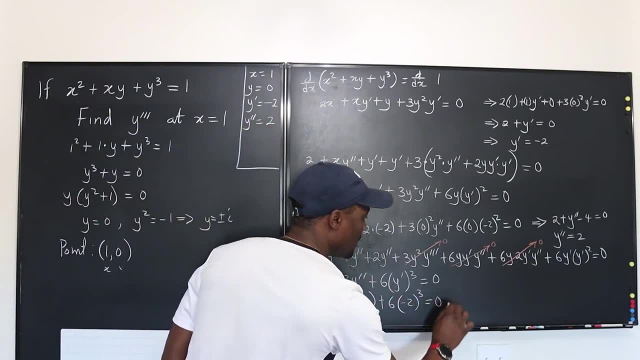 What is y prime prime? It's 2, okay, Plus 6 times. What is y prime Negative: 2, negative 2 cubed equals 0.. Ah, let's break this up here. Okay, let's do this. 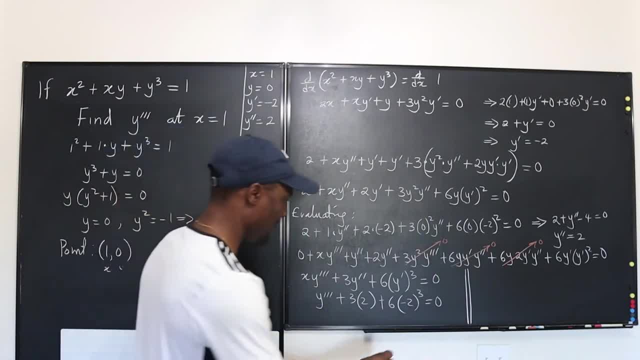 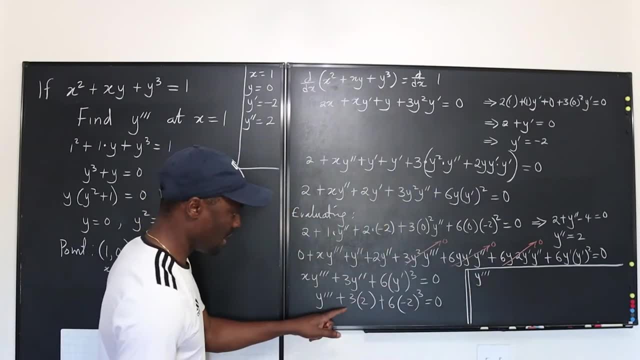 Aha, And then what we have left is that- let's put this here: We now have y, prime, prime, prime plus 6. This is going to be negative 8.. Yeah, Negative 2 cubed is negative 8, times 6 is negative 48,. okay. 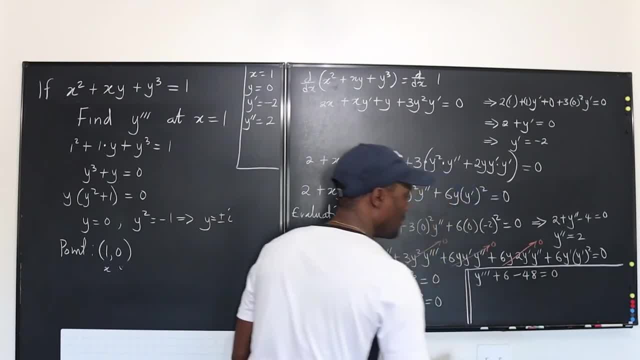 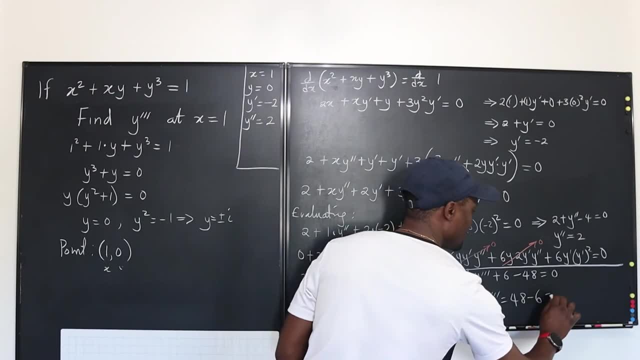 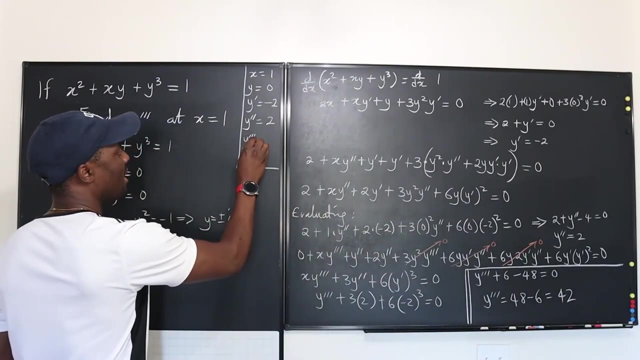 Minus 48 equals 0. That tells you that y prime prime prime equals 48 minus 6,, which is equal to 42. So we can come here and say y prime prime prime equals 42. Do you see how much dedication. 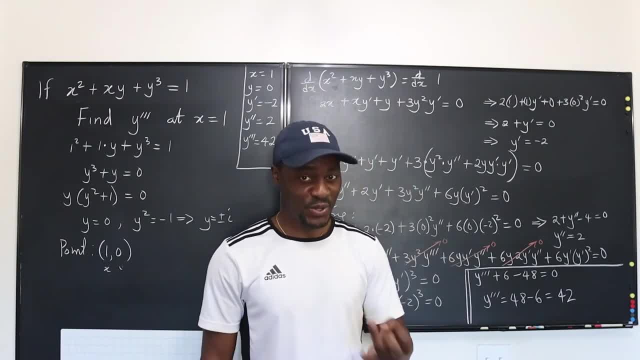 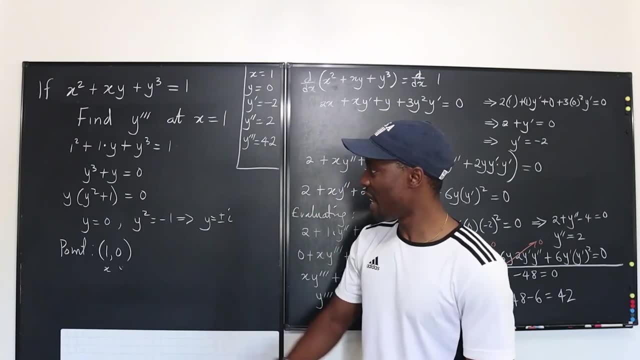 How many times you have to use the composite rule, or what you call the chain rule, and how many times you have to use the product rule When you're doing this kind of problems. you want to evaluate, you want to use the numbers. 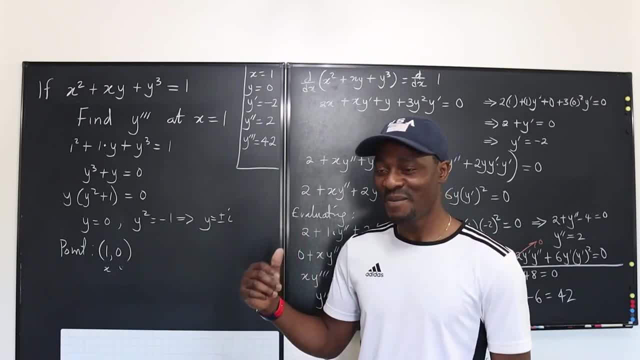 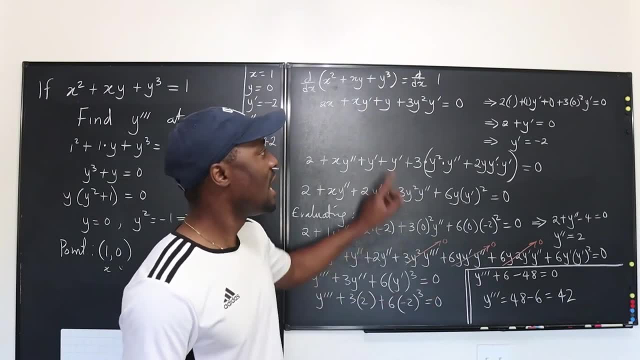 because they're going to save you at the end. Don't wait till the end, because they build up. You can just do the differentiation all the way to the last one, but when you want to evaluate, you have to go back to each of the equations that you created to evaluate each. 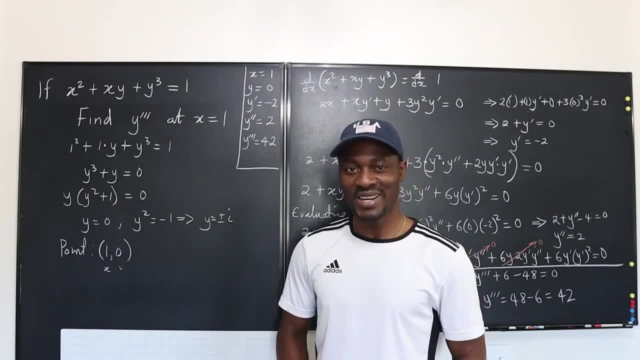 of the derivatives, Never stop learning. Those who stop learning have stopped living. Bye, bye.